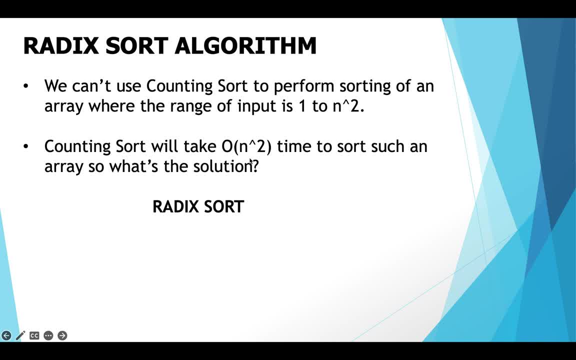 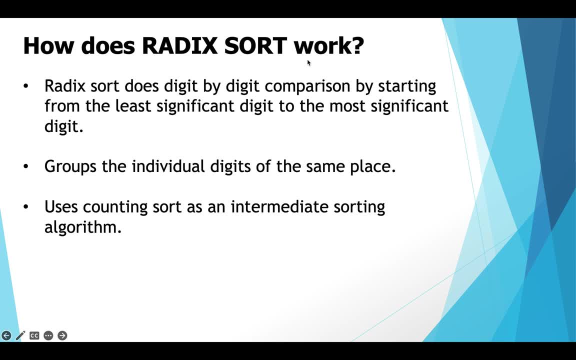 sort the array in big O squared time. So what's the solution? if we want to sort such an array, It's radix sort. So how does radix sort work? Radix sort does digit by digit comparison by starting from the least significant digit to the most significant digit: It groups. 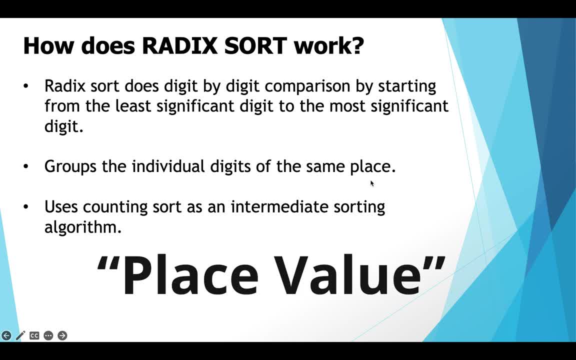 the individual digits of the same place value. Now, if you remember the phrase place value with radix sort, you will never forget this algorithm. Important thing to note is that radix sort uses counting sort algorithm as an intermediate sorting algorithm to perform sorting. This is why you should watch the video that I have made explaining the counting sort algorithm. 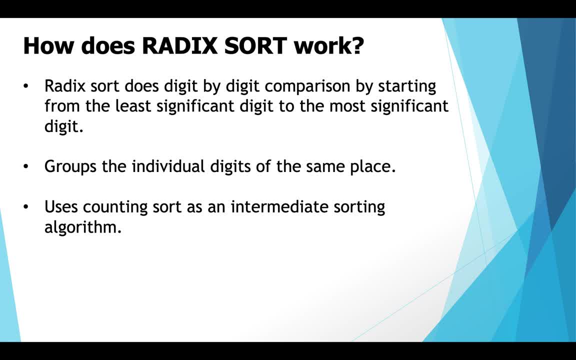 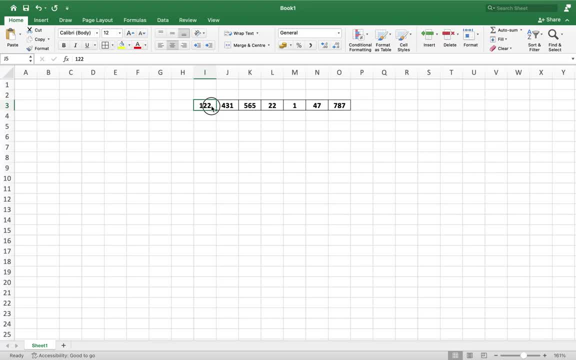 You will find the link in the description box of this video, or you can simply watch it by clicking on the i button. Let's now start understanding how the radix sort algorithm works. This is our problem array that we are going to sort using the radix sort algorithm. From this array we 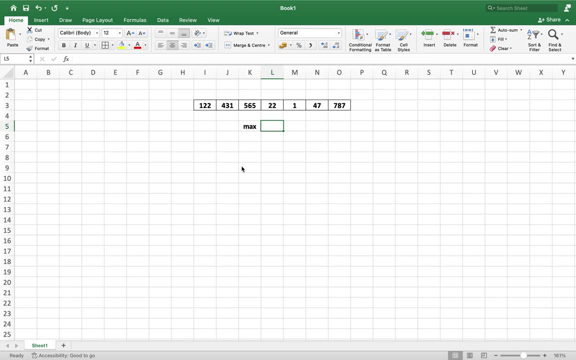 are going to first pick out the maximum element. So what's the maximum element of this array? It's 787.. Now we are going to find out how many digits does 787 have, or the maximum element of this array have? So 787 has three digits. okay, So we need to perform sorting three times on the entire. 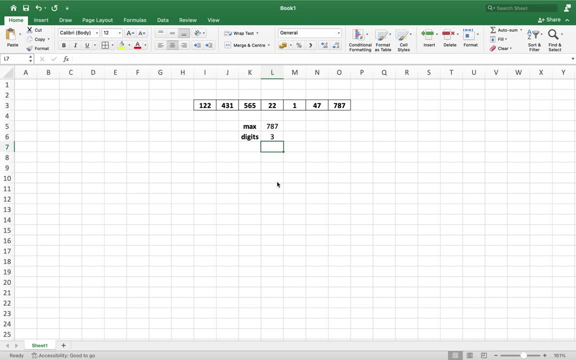 array as part of radix sort algorithm, up to the hundredths place. So we need to go through each significant place one by one. We will use the counting sort algorithm to sort the digits at each significant place. However, we need to go through each significant place one by one. We will use the counting sort algorithm to sort the digits at each significant place. However, 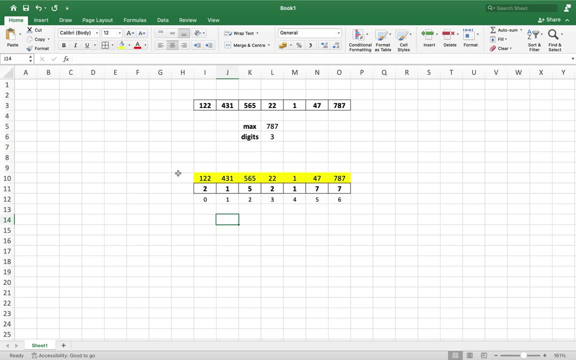 you can use any stable sorting technique to sort them, So this is the right setup to perform the sorting of the last digit of every element. The array contains the last digit or one's place of every number written above their respective cells and the number beneath the cells of the. 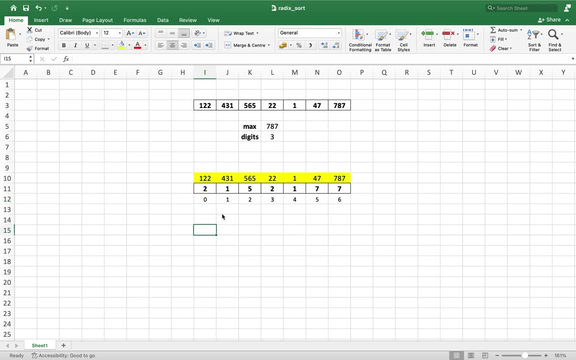 array represents the indexes of the items, Since we are using the counting sort algorithm. hence we need to create an auxiliary array Now. its size will be one plus the max element of this array. The max element of this array comes out as seven, So the size of the aux array will be 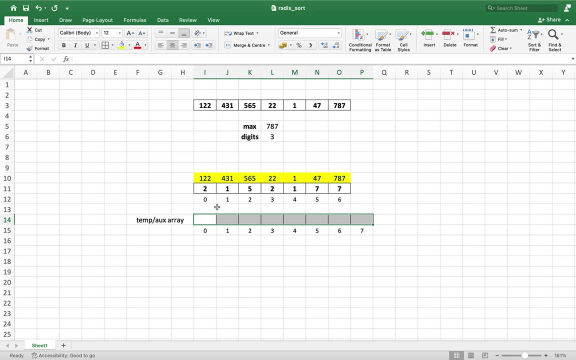 8.. Now let's quickly store the count of each element of this array into the aux array. First I am going to fill this aux array with zeros. okay, Now, the first element here is 2.. So at index 2 I increment the value by one, So the value here becomes 1. then I have 1 as the second element. 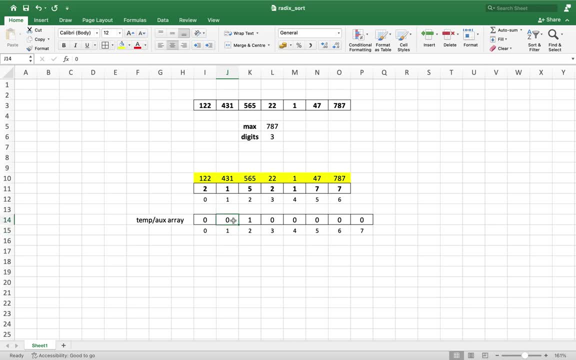 So at index 1 I incremented the value one again, and this value also becomes one. the third element is five. so the value at index five also gets incremented by one and it becomes one. the fourth element of this array is two. so at index two i am going to increment the value, which is one already, by 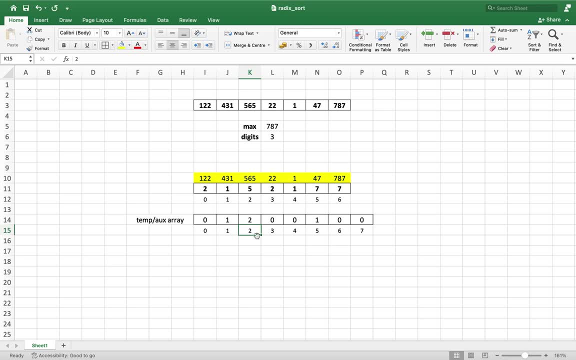 one, so this value becomes two. this means that two is present two times in this array. now the fifth element is one, so at index one i am going to increment the value by one again, so it becomes two. at index five i have seven, so i am going to go at index seven of the. 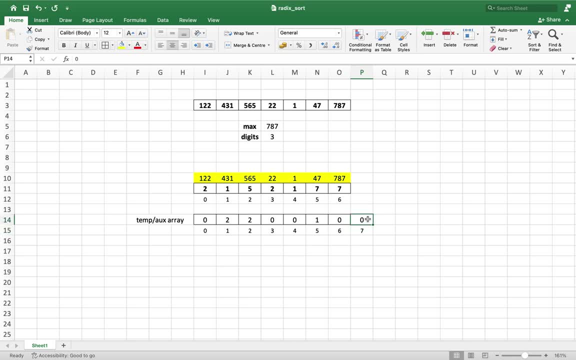 temp array and increment the value stored by one, so this becomes one again. at index six i have seven again, so i go to index seven in the temp array and increment the value stored by one, so this becomes 2. this means that 7 is present two times in the input array. 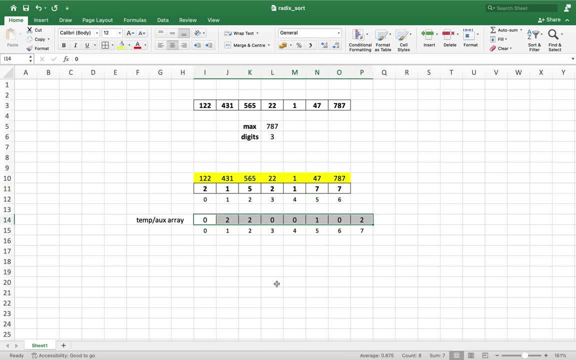 now we are going to modify the temporary array, the temporary count array, to store the cumulative sum. each element will store the sum of the previous counts. so we are going to start from this element at index 1, 2 plus 0 is going to give us 0, so no change over here. then we are going to move to this element. over here we have. 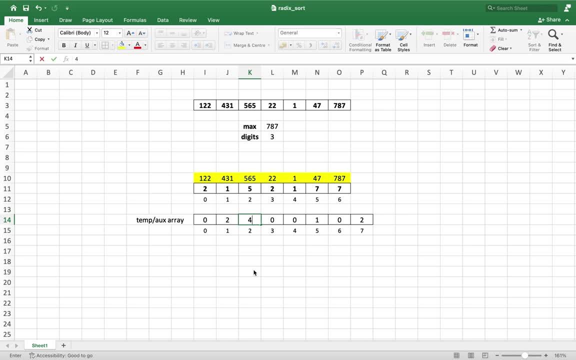 2, 2 plus 2 is 4, so I am going to put 4 over here. then at index 3 we have 0, so 0 plus 4 is going to give us 4, so let me populate 4 over here. at index 4 we have 0. again, 0 plus 4 gives us 4, so I am. 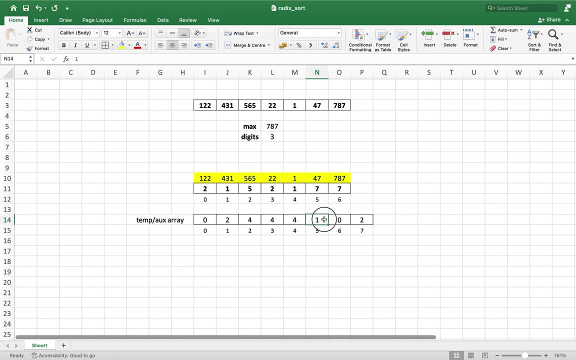 going to populate 4 over here at index 5. we have 1. 1 plus 4 gives us 5, so let me populate 5 over here. over here it will be 5 populated at index 6, and over here, 2 plus 5 is going to give me 7. 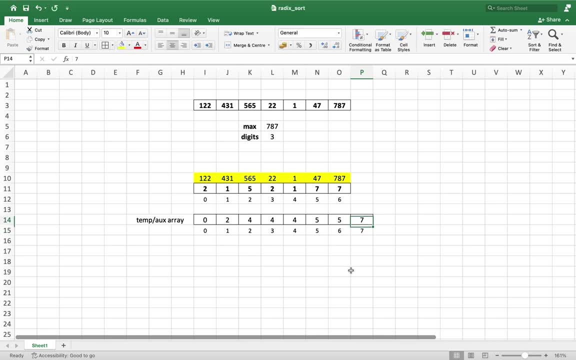 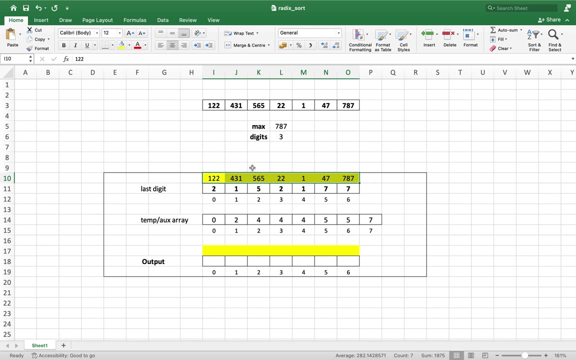 so 7 will be populated over here at index 7 in the temporary count array. so the array has now been modified to provide us the position of each element in the output sequence. so the next step is going to sort the numbers based on the last digit in counting sort. 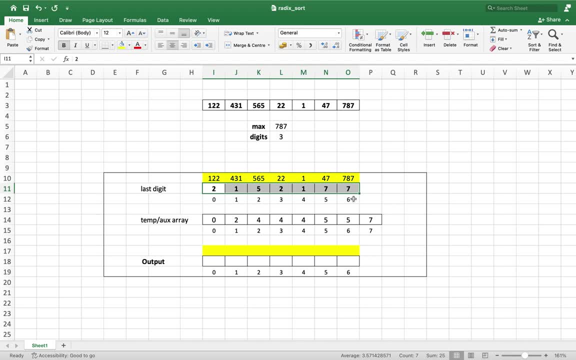 we start from the left and go towards the right, but in this case, we are going to start from the right and go towards the left. why? because these repeating digits, they represent different numbers and we want to place them correctly in order to sort them properly. so we are going to start from. 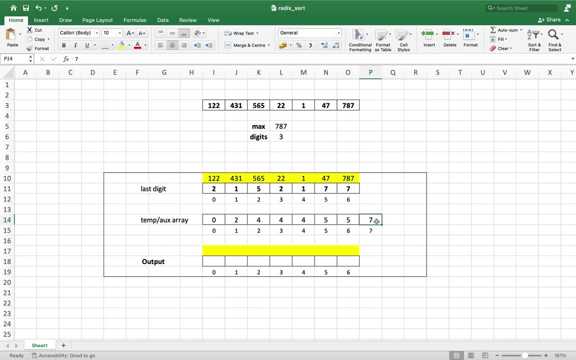 the right. the value here is 7. so we go to index 7. here we find 7. we subtract 1 from it, so we get 6. we update 6 over here and at index 6 we place 7 and the corresponding number, which is 787. then we 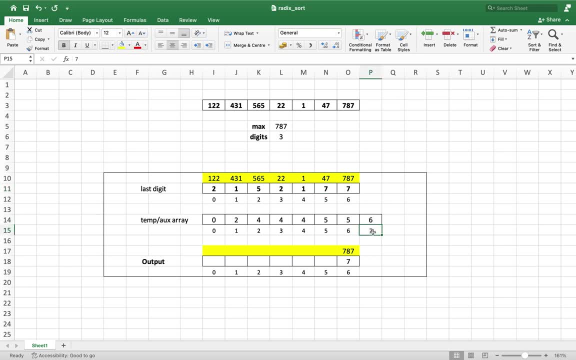 go to the next element. over here we have 7. we go to index 7, we find 6 over here. we subtract 1 from it, we get 5. we update this item with 5. at index 5 in the output array we place 7 and the. 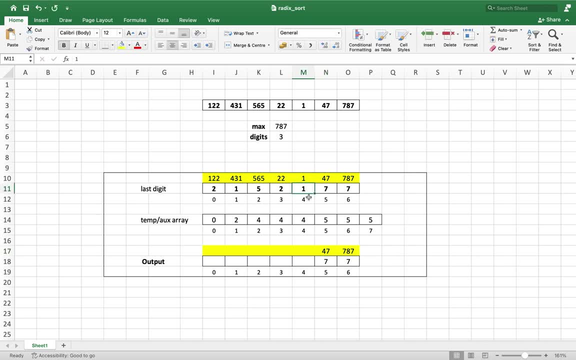 corresponding number, which is 47. then we go to the next element, which is 1. so we go to index 1. we find 2 over here. we subtract 1 from it, we get 1. we update this item over here with 1 and at index. 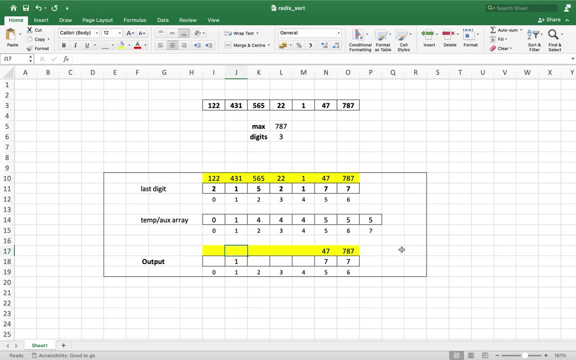 1. we place 1 and the corresponding number, which is 1, we go to the next element. here. we have 2. we go to index 2. we find 4 over here. we subtract 1 from it, we get 3. we update 3 over here and 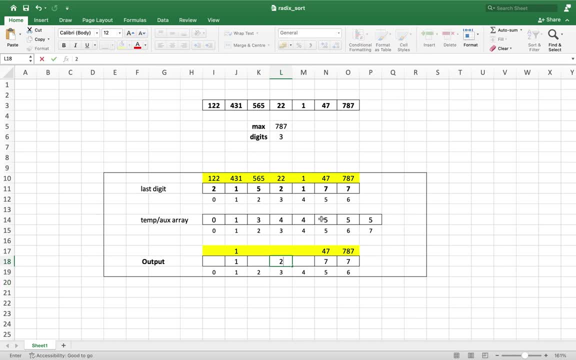 at index 3 we place 2 and the corresponding number, which is 22. okay, then the next element is 5. so we go to index 5. we find 5 over here. we subtract 1 from it, we get 4. we update this item. 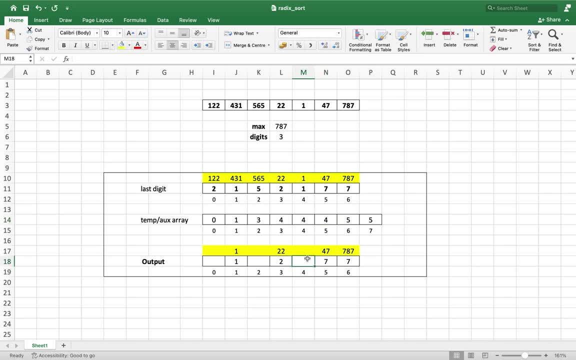 with 4, and at index 4 we place 5 and the corresponding number, which is 565. then the next element is 1. we subtract 1 from it, we get 0. we update 0 over here and at 0 we place 1 along. 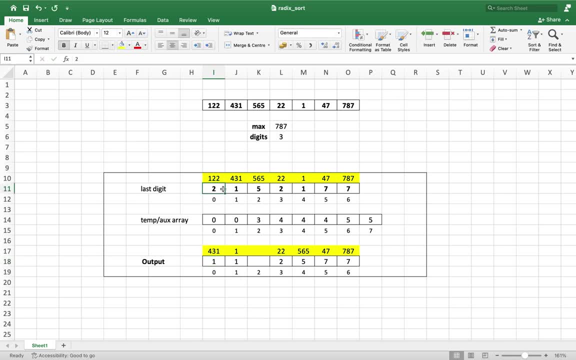 with the corresponding number, which is 431, and the last element is 2. so we go to index 2, we find 3 over here, we subtract 1 from it, so we update this item with 2 and at index 2 we place 2 and the. 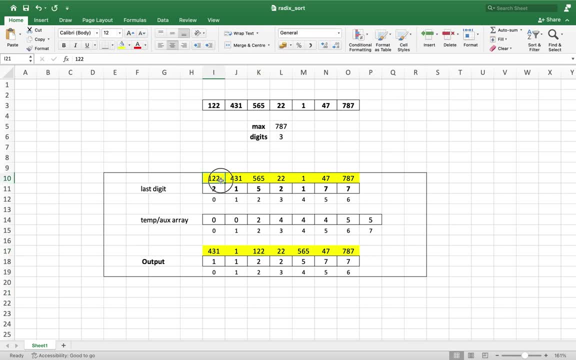 corresponding number, which is 122. all right, so this array is sorted using counting sort algorithm. last digits, that means once place. okay, now we are going to sort this intermediate output array based on the tens digit, that means the middle digit. so this is going to be our input array. 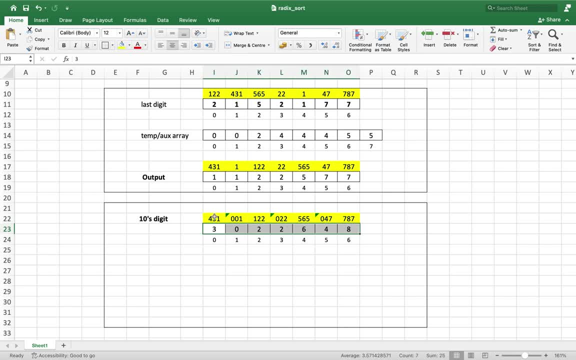 and you can see I have placed the middle digits of these numbers over here. okay, now we are going to sort this array based on the middle digit or the tens place. okay, so we are going to first create a temp account array, as we do in counting sort algorithm, the. 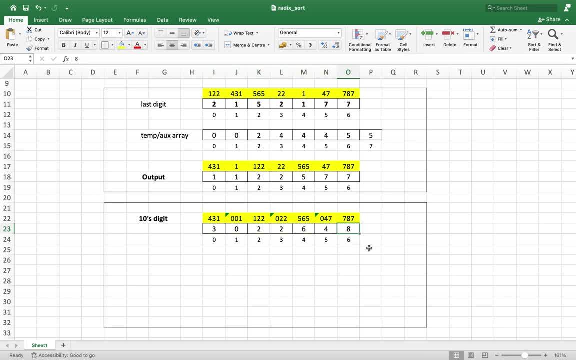 maximum element from this array comes out as 8. so we are going to create a temporary count array of size 9.. now let me quickly fill this array with the counts of the respective elements from this array. before that, I am going to fill this array with zeros. now let me start from the first element. 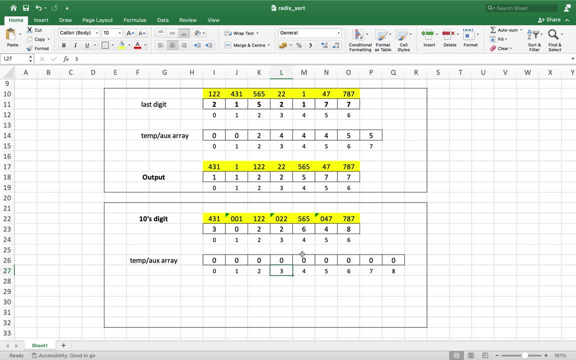 we have three as the first element, so we go to index three. here we increment the value by one, so this value becomes one. the next element is zero. so we go to index zero. here we have the value zero, we increment it by one, so we get one over here, over here we. 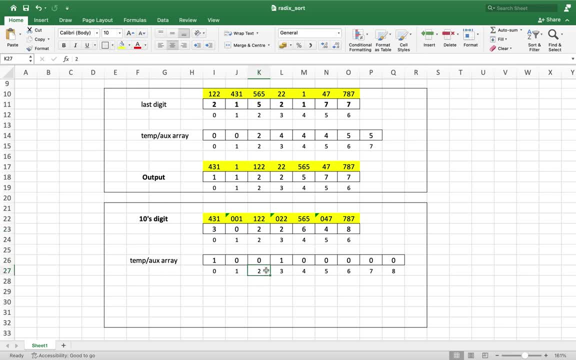 have two, which is the third element. so we go to index two and we increment the value by one, so we get one over here. the fourth element is two, so we go to index two. here we have one, we increment it by one, and then the fifth element is six. so we go to index six, where we have zero, we incremented by. 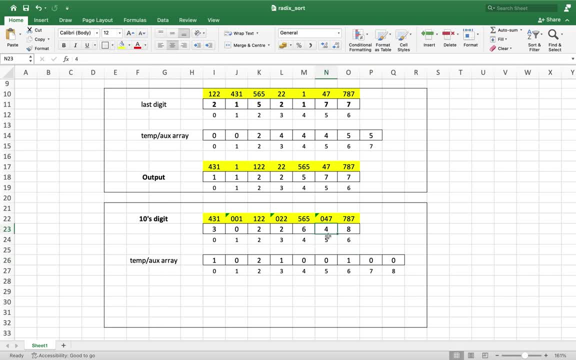 one, so the value here becomes one. over here we have four, so we go to index four. here we have zero. we increment it by one, so let me place 1 over here, and the last element is 8.. so we go to index 8. here the value is zero. we increment it by one, so the value here becomes one. 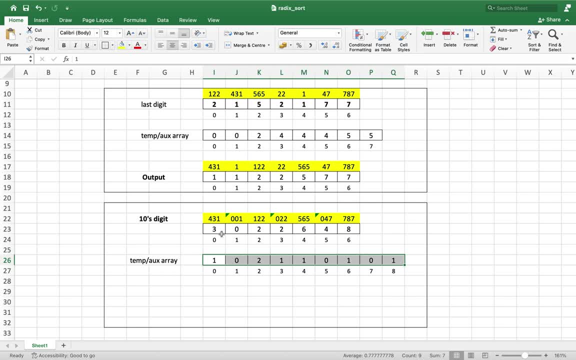 the temporary count array now holds of the respective elements of this array. now let's modify the temporary count array to store the cumulative sum, as we did over here. so we are going to start from this element. the value that this index is going to get will be 0 plus 1, so it will be 1. over here it will be 2 plus 1, so it. 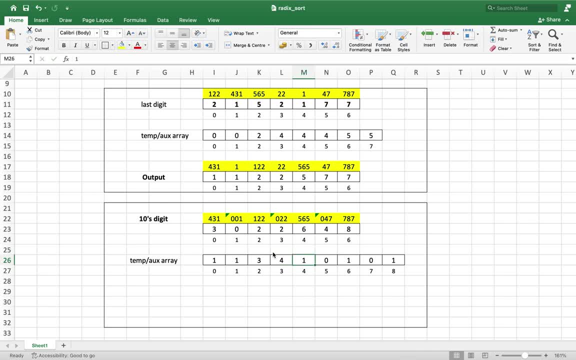 will be 3. over here it will be 4. then the value here is going to be 4 plus 1, which is 5. so let me place 5 over here. it will be 5. over here it will be 6. in this cell of the array it will be 6, and. 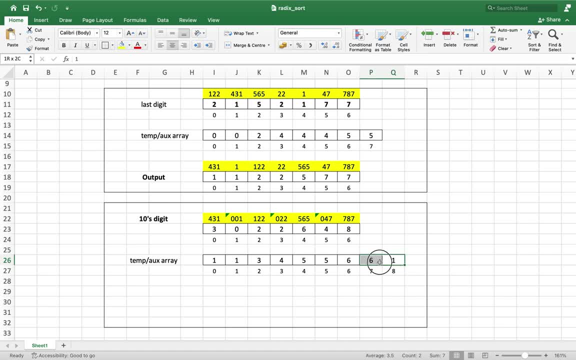 in the last cell of the temporary count array, the value will be the addition of 6 and 1, so it will become 7. all right, now let's perform the final step, which is going to sort this array based on the tenth digit. so we are going to start from this element, which is 8, so we go to index 8 here. 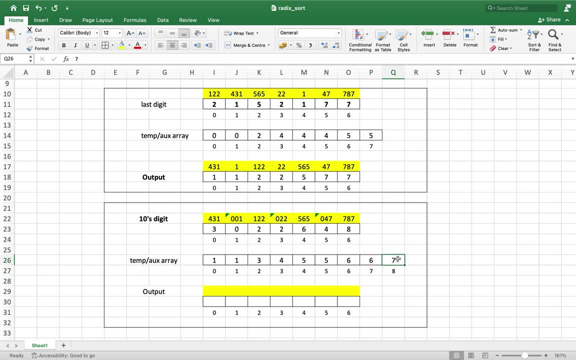 we find 7. we subtract 1 from it, we get 6, so we update 6 over here. and at index 6 we place 8 and the corresponding number, which is 787. then the second element from the right is 4. so we go to index 4. we find 5 over here. we subtract 1 from it. we get for, so we update. 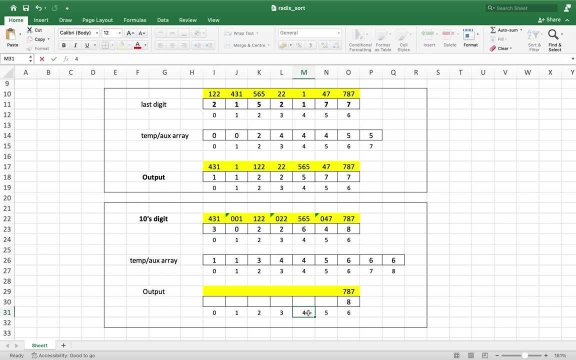 this cell with 4 and at index 4 we place 4 and the corresponding number, which is 47. then the third element from the right is 6. so we go to index 6. here we find 6. we subtract 1 from it, we get 5. 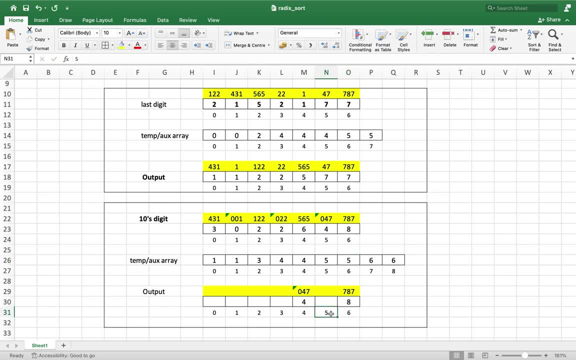 we update this cell with 5 and at index 5 we place 6 and the corresponding number, which is 5, 6, 5. the fourth element from the right is 2. so we go to index 2. here we find 3. we subtract 1 from it. 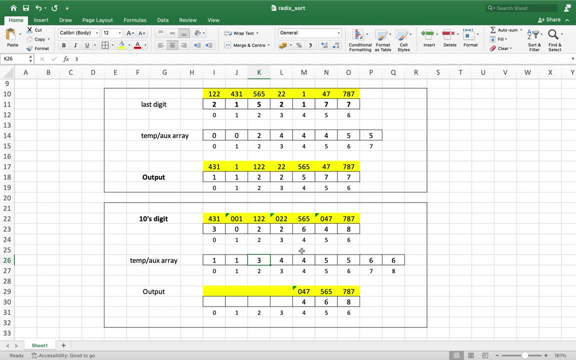 we get 2, so we update this cell with 2 and at index 2 we place 2 and the corresponding number, which is 0 to 2. okay, the next element is 2, so we go to index 2 again. here we find 2. we subtract: 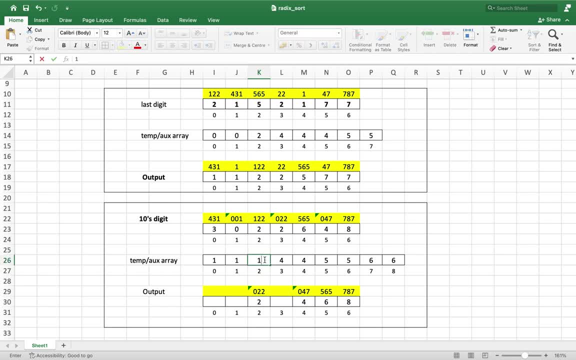 1 from it. so we get 1. we update the cell with 1 and at index 1 we place 2 and the corresponding number, which is 1 to 2. okay, now the next element is 0, so we go to index 0. 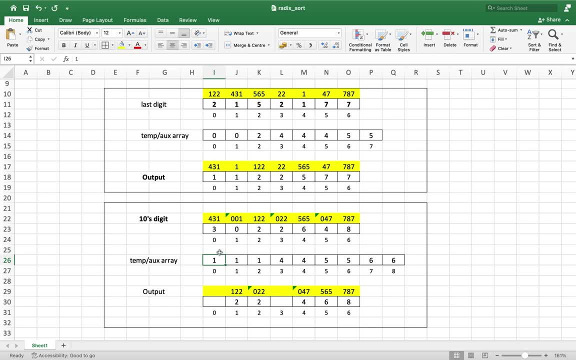 here we find 1, we subtract a 1 from it, so we get 0. we update the cell with 0 and at index 0 we place 0 and the corresponding number, which is 1. all right now, the final element is 3, so we go to. 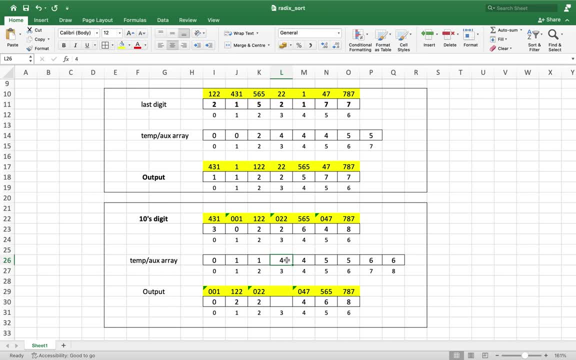 index 3: here we find 4. we subtract 1 from it, we get 3 and the corresponding number, which is 2. so at index 3 we place 3 and the corresponding number, which is 4, 3, 1. all right, and there you go. 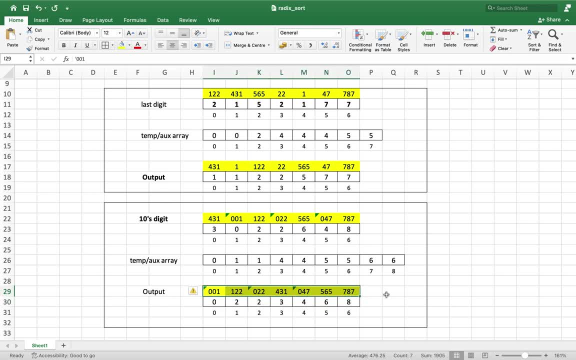 the array is sorted based on the 10th digit. so first this array was sorted based on one's place and then it got sorted based on the 10th place, all right, or the middle digit. now this is an intermediate output array that we are going to sort based on 100s place or the leftmost digit. 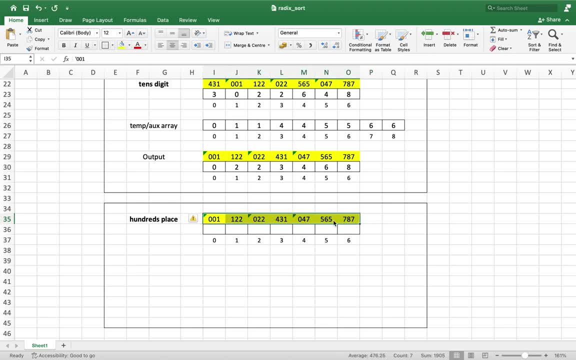 now the counting sort algorithm is going to run for the third time and this is going to be the input array. technically, the input array is going to be the digits at 100s place of these numbers. all right, so the maximum element from this array is 7, so we are going to create a temporary count. 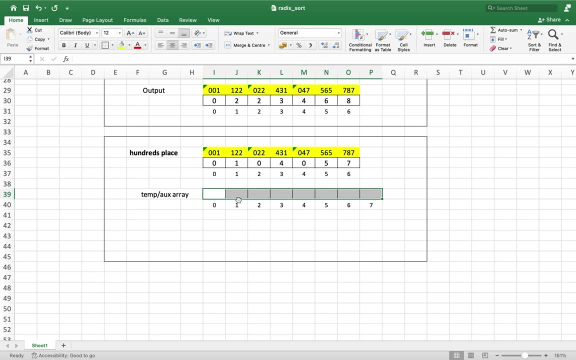 array of size 8, and let me fill this array with sorry sorry, and let me fill this array with sorry Zeros. now we are going to store the count of each of these elements in this array, So we are going to start from this element. here We have 0, so at index 0. 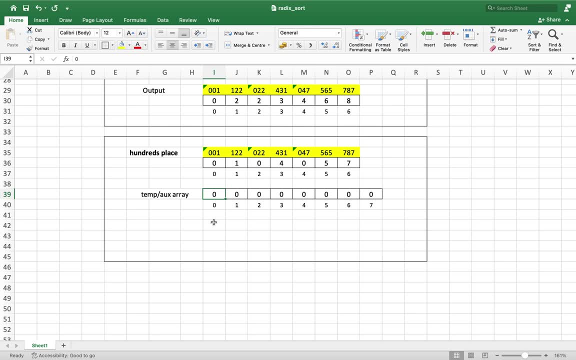 We are going to increment the value stored, which is 0. we increment it by 1, we get 1, so we update the cell with 1. The next element is 1, so we go to index 1 here. We increment the value by 1. 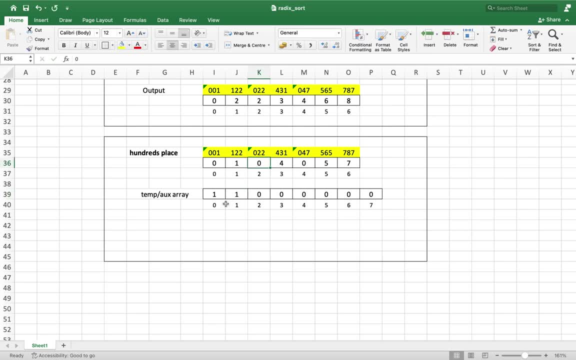 So this value becomes 1. the next element is again 0, so we go to index 0. here We have 1 already. we increment it by 1, it becomes 2. the fourth element is 4, so we go to index 4. here The value is 0, we increment it by 1, we get 1 and we get 0 the third time. 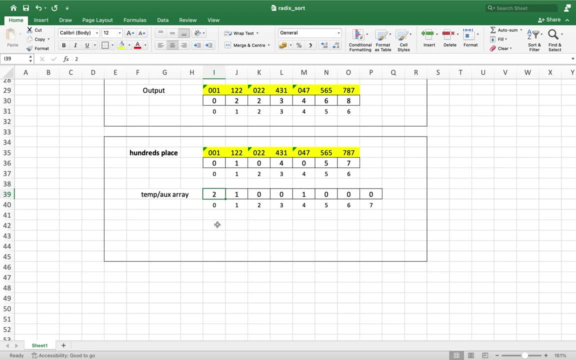 so we go to index 0. here we have 2, we increment it by 1, we get 3, and The second last element is 5. so we go to index 5. here The value becomes 1, 0 plus 1 is 1, and finally we have 7. so at index 7 we have: 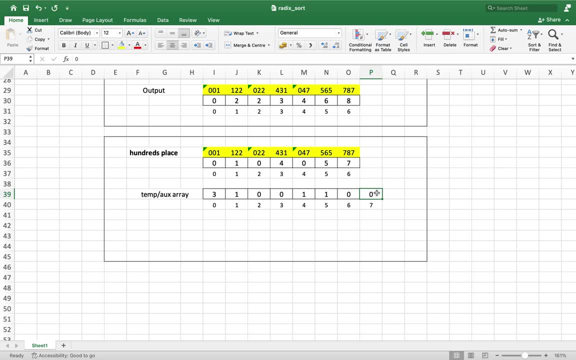 1.. That will mean we have carried out a criticism and we have change 4, So the differentiating value as the change will be of 0 value as 0 we incremented by 1, So this cell will hold 1 as its value. Now let's modify this temporary count array. 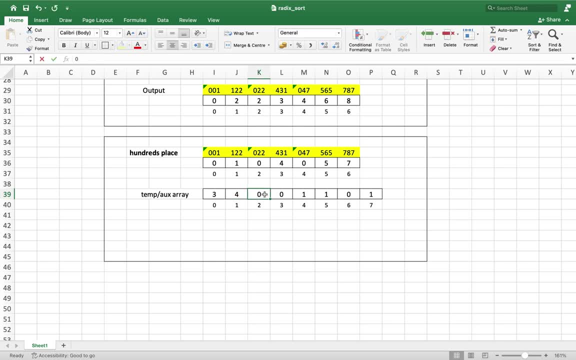 To store the cumulative sum. so we are going to start from this cell. We are going to add 1 and 3, so that will give us 4. so we update this cell with 4. We move to this cell. here We have 0, 0 plus 4. we update 4 over here. 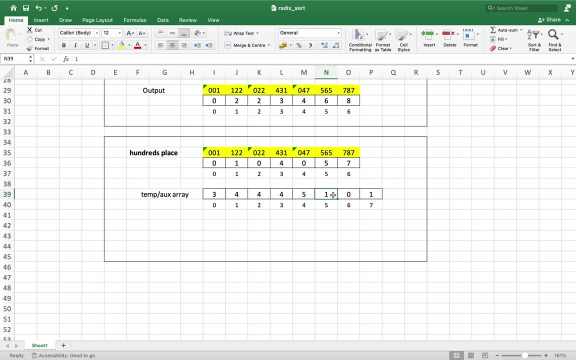 Then in the next cell We are going to update 4, because 0 plus 4 is 4. in the next cell it will be addition of 1 and 4, so be 5 over. here it will be the addition of 5 and 1, so it will be 6 over. here it will be the addition. 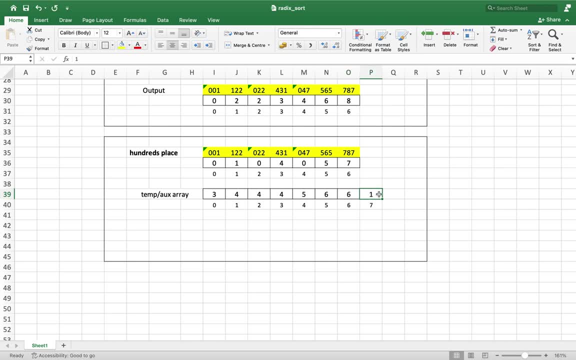 of 0 and 6, so this will be 6, and the last cell is going to hold the addition of 1 and 6, which is 7, so i place 7 over here. all right, now let's perform the final step in which we are going to sort this. 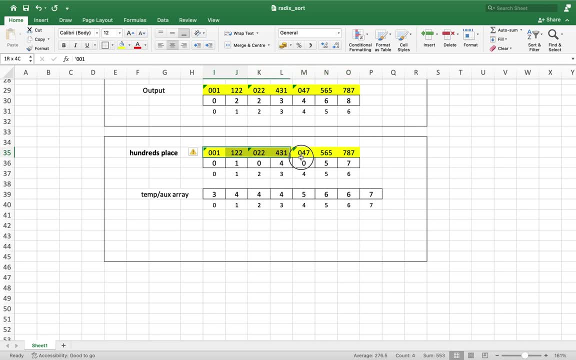 array by hundreds place and basically this will be the final sorting step that is going to sort this entire array in ascending order. so we are going to start from the rightmost cell and move towards the left. so the first cell when we start from the right is 7. so we go to index 7. here we 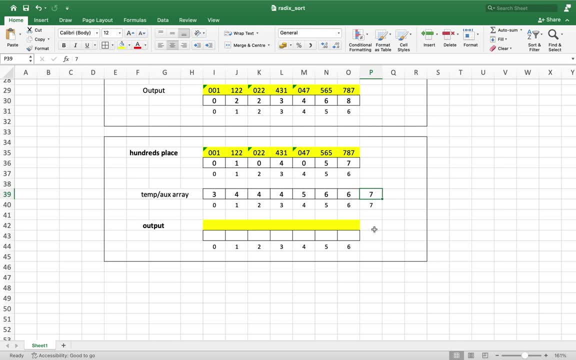 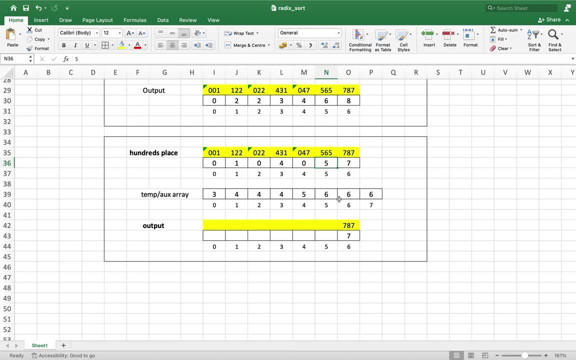 second element from the right hand side. here we have 5. so we go to index 5. here we find 6. we subtract 1 from it, we get 5. we update this cell with 5 and at index 5 we place 5 and the corresponding. 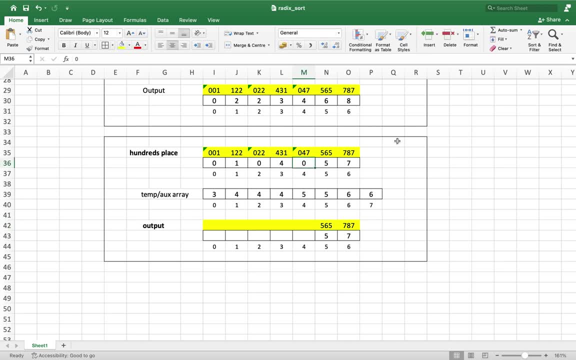 number, which is 565. then we go over here, we get 0. now we go to index 0, here we find 3, so we subtract 1 from it, we get 2. so we update 2 over here and at index 2 we place 0 and the corresponding number. 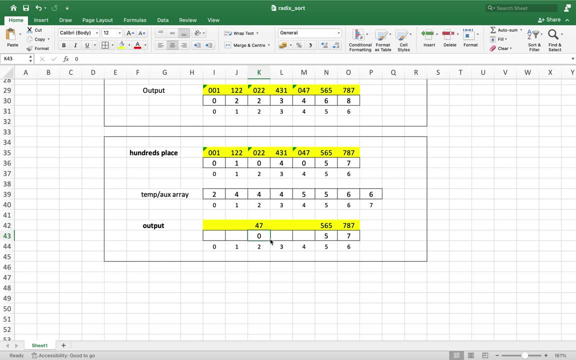 which is 47. let me place 47 like this now. and the next element is 4. so we go to index 4. here we find 5. we subtract 1 from it, we get 4. so we update this cell with 4 and at index 4 i place 4 and the. 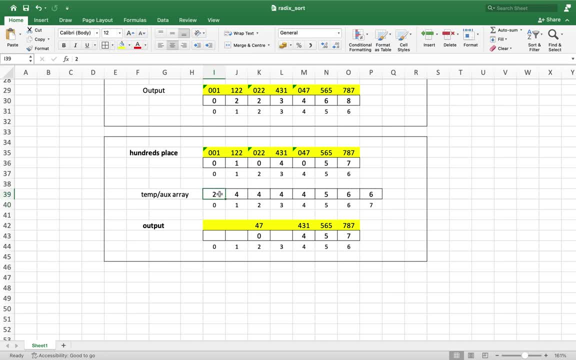 next element is again 0, so we go to index 0. here we find 2, we subtract 1 from it, so we get 1, which we update over here, and at index 1 we place 0 and the corresponding number, which is 22. okay, then the next. 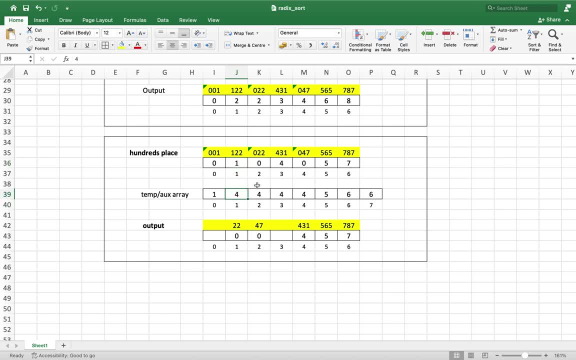 element is 1. so we go to index 1. here we find 4. we subtract 1 from it, we update this cell with 3, and at index 3 we place 1 and the corresponding number, which is 1 to 2, and the final element is 4. so we 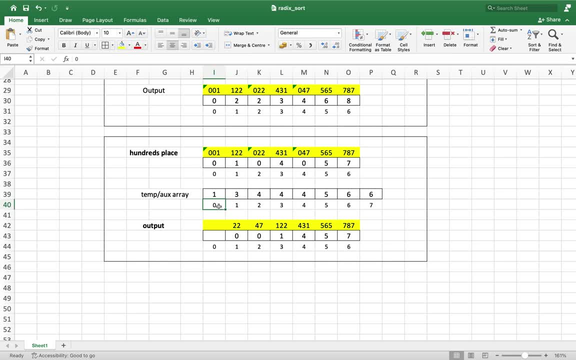 go to 0th index. here we find 1, we subtract 1 from it, we get 0. we update this cell with 0 and at index 0 we place 0 and the corresponding number, which is 1, and there you go, the array is sorted. 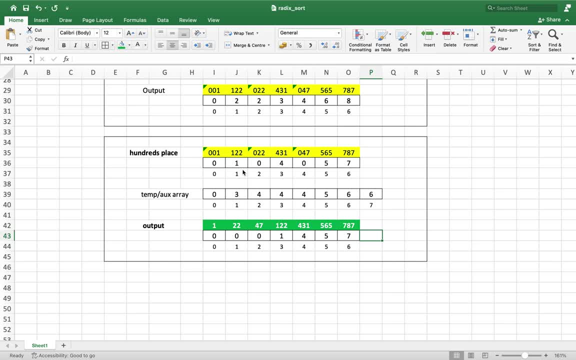 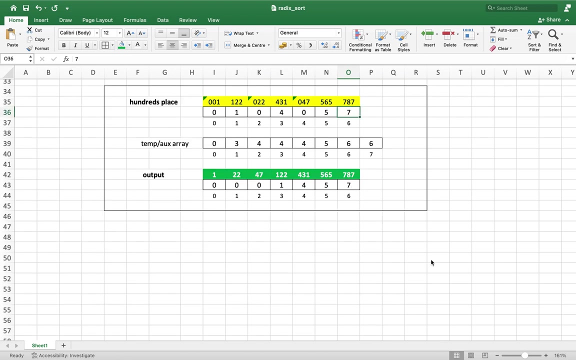 now in this case, especially if i had started from the leftmost element and had moved towards the rightmost element, i would have placed this one over here at the third cell, which would have been wrong. this is why it's very important that we start from the right hand side and move towards the left hand side now. 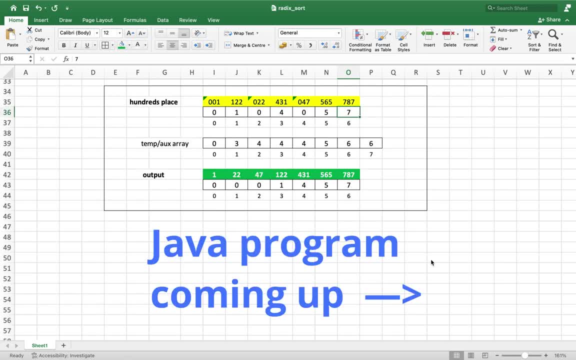 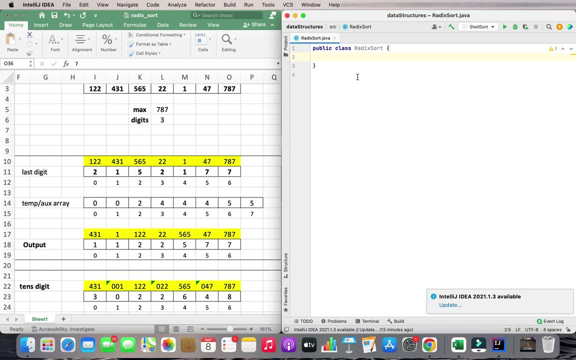 let's implement the reddick sort algorithm in a java program, because that is going to teach you how to write the reddick sort algorithm in the first place. here i am in my intellij ide, where i have created this class, reddick sort, in which i'm going to create: 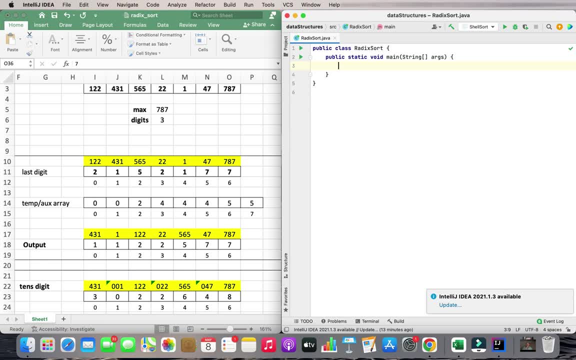 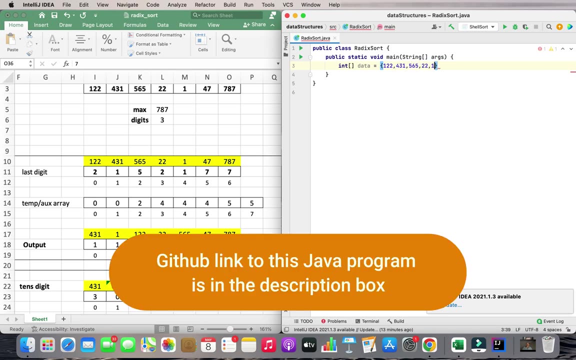 first, the main function in which i'm going to first declare and initialize an array, so let me call it data, and it's going to contain a few elements which will be 122, 431, 565, 22, 147, 787. now let me create the object of this class which i'm going to use to call the reddick sort function, so let me. 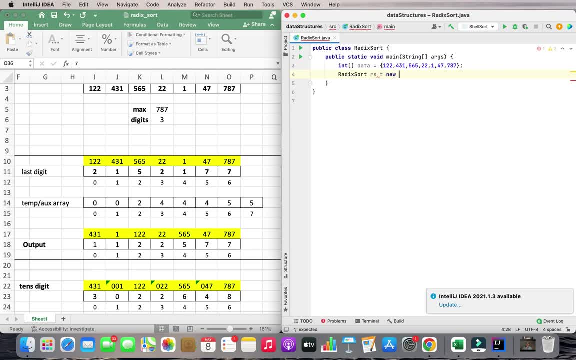 create the object. i'm going to call it rs, all right, and i'm going to use this rs object to call the reddick sort function, and the parameters that i'm going to pass to this function will be the array, so it will be data and the size of the. 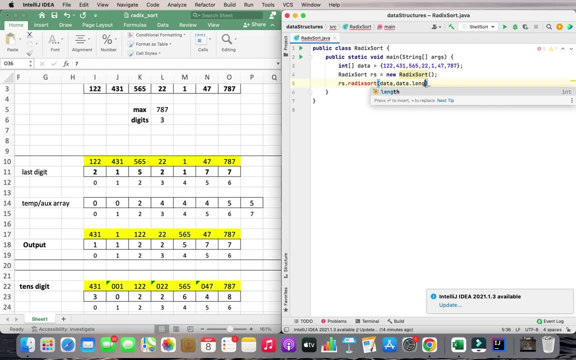 array or the length of the array, so it will be data dot length. i haven't created the function yet. that's why it's highlighted in red. i would also like to print the array before calling the reddick sort function and after calling the reddick sort function. so let me call it rs object and i'm going to. 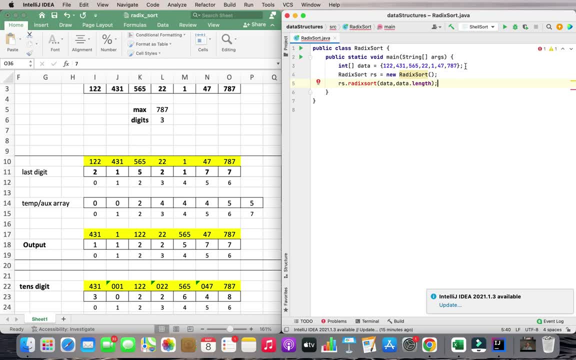 call the array into the array. so that's why it will get a setting of rs object: andzelan vé Brush. so i'm going to take the array and i'm going to are all the array and i'm going to. Christians all also see that the array, array, the array sets this up. all the ler llam call here. 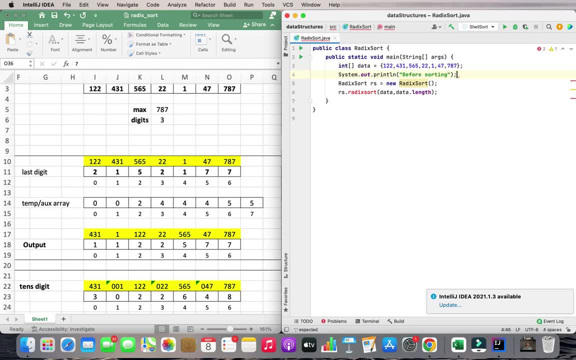 and i'm going to call them aBoly, and brings up the array. so if i бр Mov-Enter, i'm going to ask mysti in here, m on my team, and then i'm going to write here: loop* T işte. and then i'm going to bring up mystate. 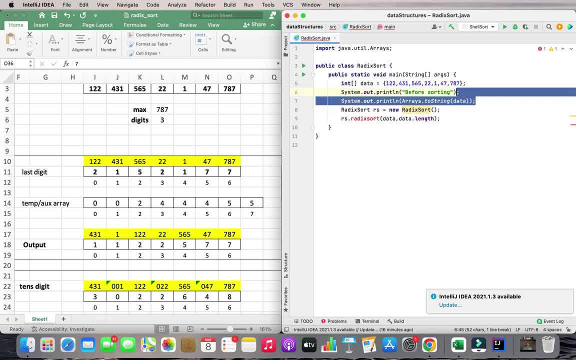 called affix, going to copy these two lines of code and paste it after the call to the reddick sort function over here. i'm going to make a small change. i'll write after sort. okay, so this line of code is going to print the problem array and this line of code is going to print the sorted version of the. 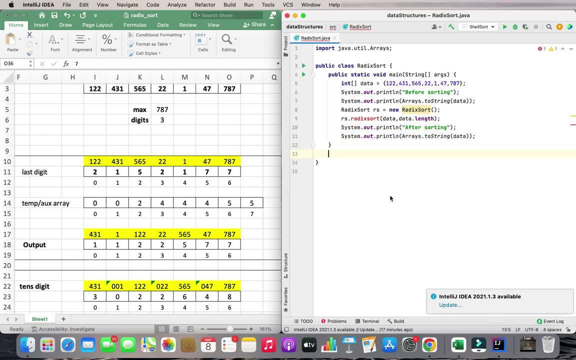 array sorted using the reddick sort algorithm. now let's create the reddick sort function, so it will be void reddick sort, and it's going to accept an array as the first parameter and it's going to accept the size of the arrays, the second parameter. all right, the first thing that we did when we 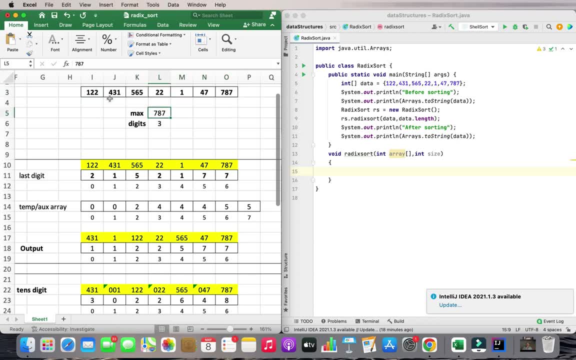 started working on the reddick sort algorithm was to find the maximum element from this problem, array. so let's write the code for that. so it will be: int. max equals to array. element that you and then i'm going to start a for loop. we'll start from index one and it's going to run for. 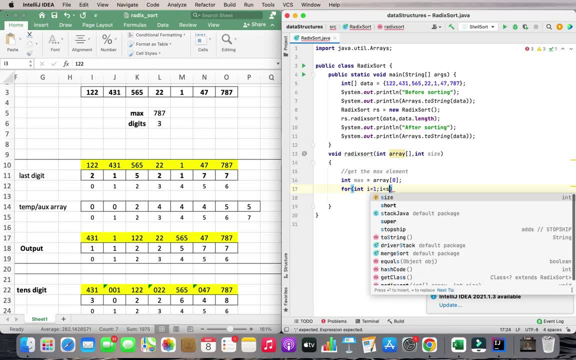 the length of the array. so i will be less than size i plus plus and within for loop it will be an if condition. if max is less than array at index i, then max will be assigned the element at index i of the array. okay, so this is the code to get the 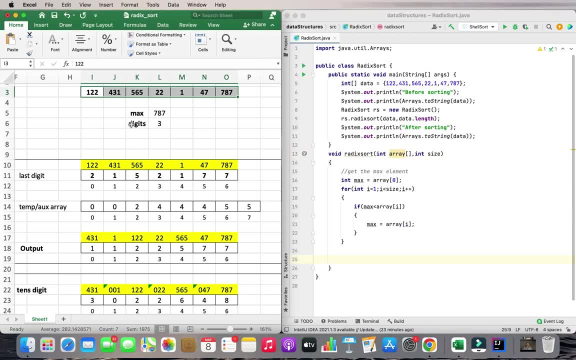 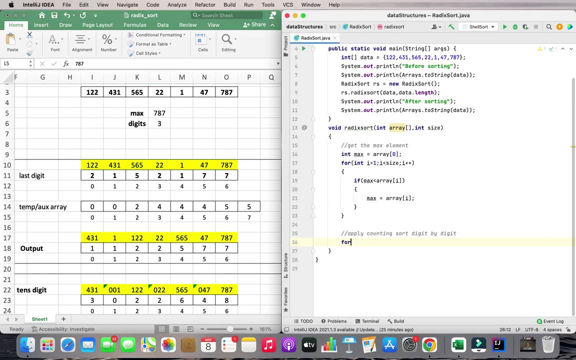 maximum element from this array. now the next step will be to apply the counting sort algorithm on this array. the counting sort algorithm will be applied three times because there are three digits in the maximum element. let's write the code for that. we are going to write a for loop, that is: 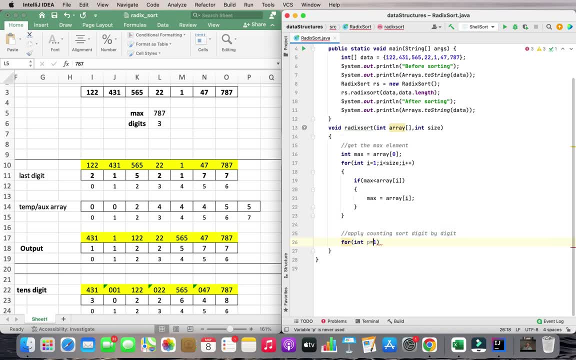 going to start from one- p represents place over here- and then we are going to write a for loop. why p is equal to one? because we'll be sorting the elements of the array first based on one's place. all right, now, the terminating condition of this for loop is going to be max. 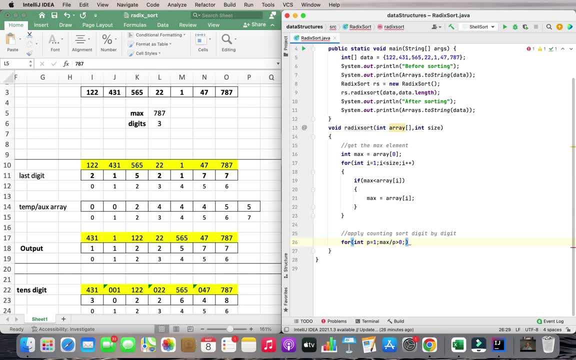 divided by p greater than zero, and the final condition is going to be: b multiplied equals to 10. so let's understand this: this loop is going to run till max divided by p is 0.. So the max over here is going to come out as 787.. 787 divided by: 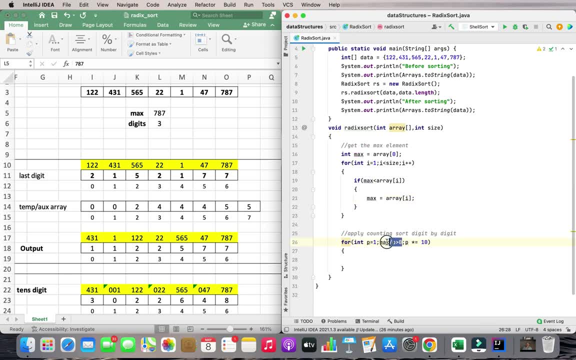 1 is going to give us 787, which is greater than 0.. So the loop is going to run, and that will be the first iteration. In the second iteration, p will become 10.. So it will be 787 divided by 10.. 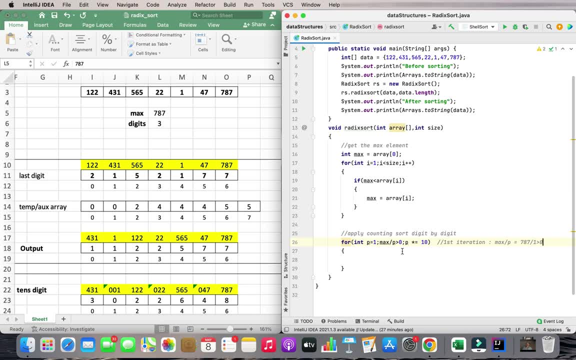 The question will be 78.. It's again going to be greater than 0. So the loop is going to run and that will be the second iteration. In the third iteration the value of p will become 100. So max by p will be 787 by 100.. The question is going to come out as 7.. The value is greater than 0.. 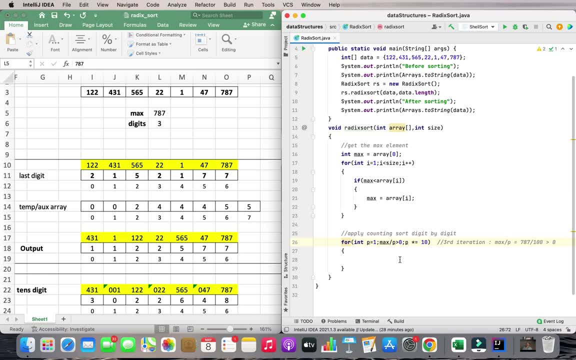 So the loop is going to run and that will be the third iteration. However, in fourth iteration the value of p is going to become 1000.. 787 by 1000 is going to yield 0, and 0 is not greater than 0.. So the loop. 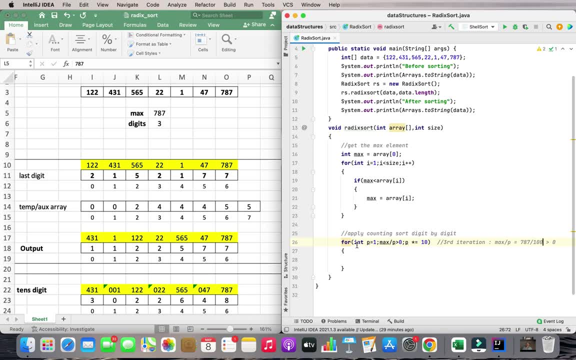 is not going to run, It is going to terminate. So now you understand the loop, Alright, and thus the counting sort algorithm will be applied three times. So let's make a call to the counting sort function. So it will be counting sort and it's going to. 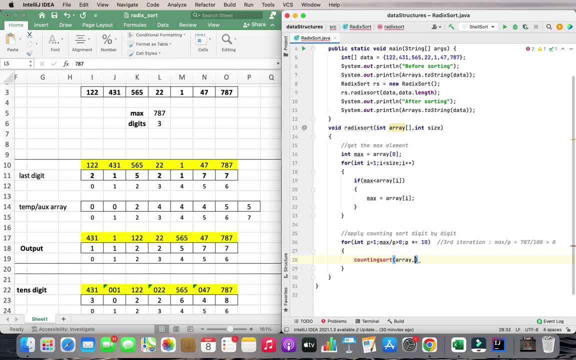 accept, obviously, array as the first parameter. The second parameter will be the size of the array, So it will be size and the third parameter is going to be p, the place That is important right Now. let's create the counting sort function. It will be white counting sort and obviously it's. 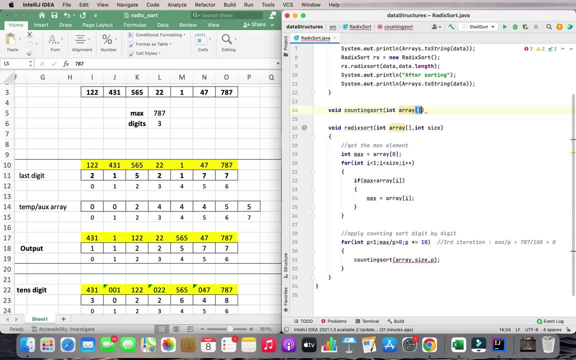 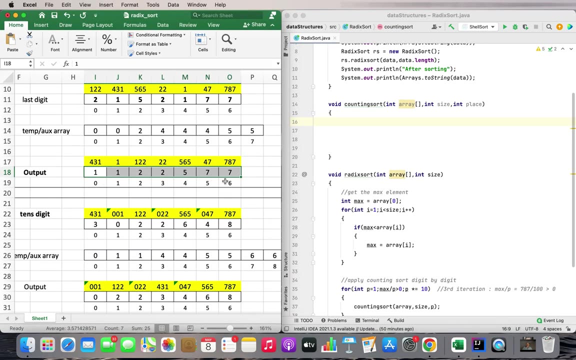 going to accept the array as the first parameter, Then it's going to accept its size and finally, it's going to accept the place based on which it needs to sort the elements. Okay, The first step will be to create the output array that will be of the same size as the input array. Okay, So I'm. 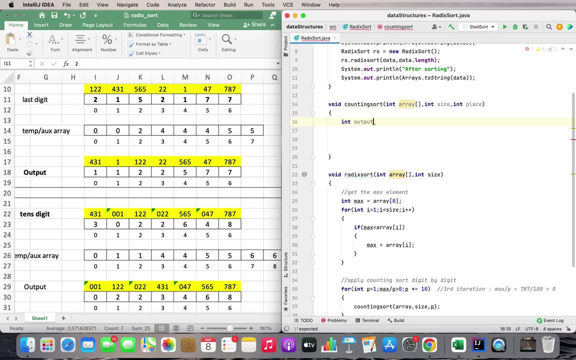 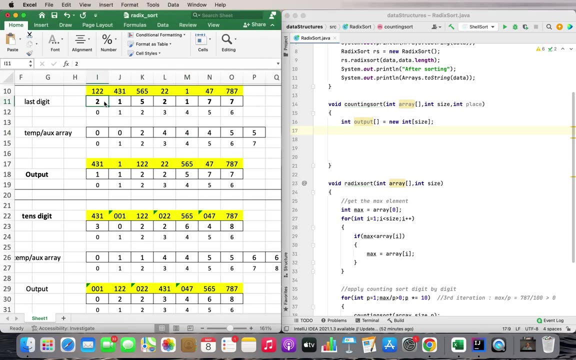 going to write the code for that. It will be int output square brackets equals to new int, and within square brackets I'm going to write size. Okay, Now. the next step will be to create the temporary count array Now, since we'll be applying the counting sort algorithm on individual digits that we are. 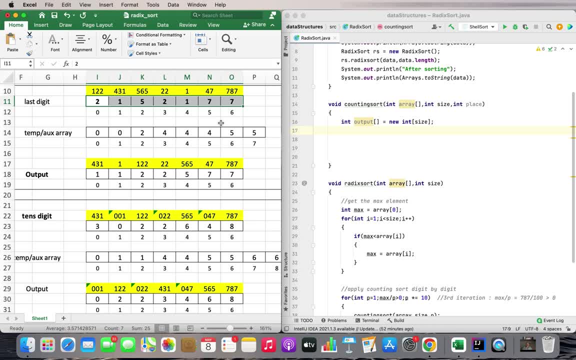 going to calculate based on ones tens and hundreds place. the individual digits will always fall in the range of zero to nine. That means the size of the temporary count array will never exceed 10.. So why not create a temporary count array of size 10 and get it over with? So let's write the code. 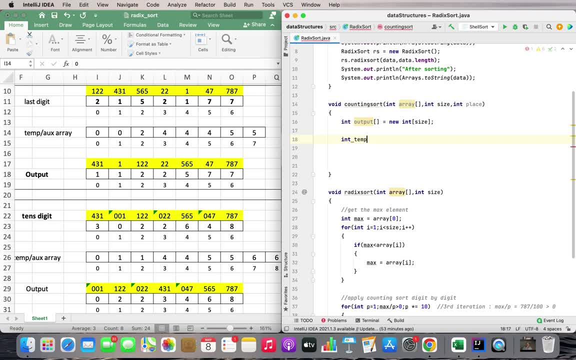 for that It will be int. temp. Temp count within square brackets equals to new int and within square brackets Let the size be 10.. Okay, Now we are going to write the code to fill the temporary count array with zeros. I'm going to 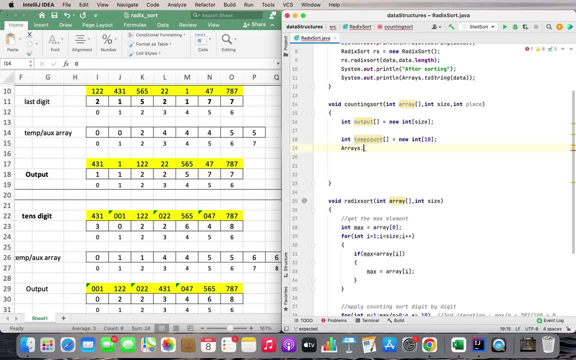 stick to writing Java code for that. So it will be arrays: dot fill. within brackets It will be the array name, which is temp count, comma zero. All right, This is going to fill the entire array with zeros. All right, Now we are going to write. 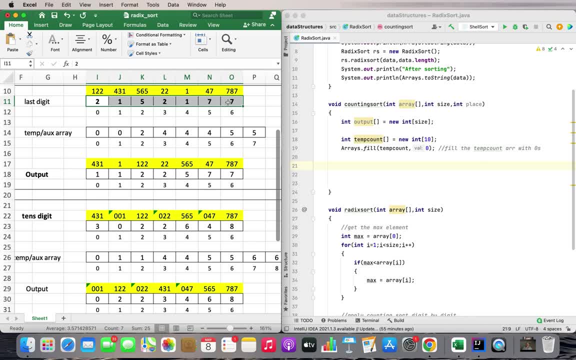 the code to store the count of distinct elements of this array into the temporary count array. So I'm going to be writing a for loop. It will be for int, i equals to zero and it's going to run for the length of the array. input array. So it will be i less than size. i increment operator. 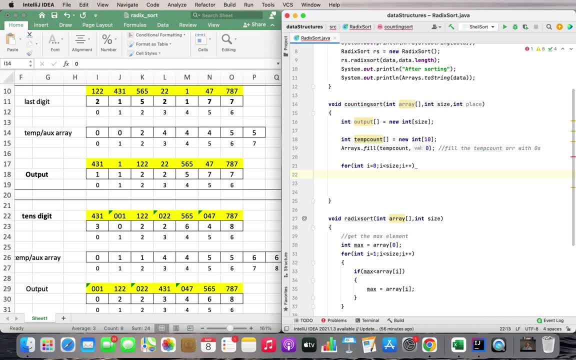 And we will be storing the count in the temporary count array, So it will be temp count and within brackets. What expression should we write? That expression, that code expression, should calculate these digits. That means the digits at one's place, the digits at 10's place and the digits 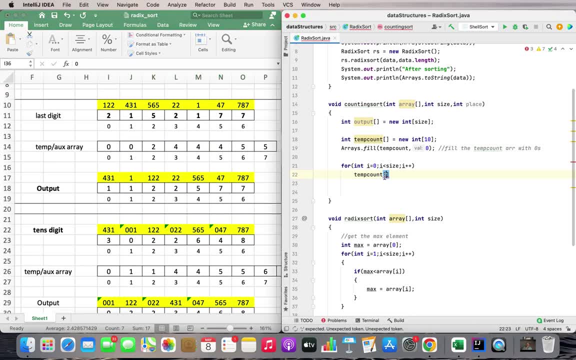 at 100's place on the code. So it will be within brackets: array at index i divided by the place variable modulo operator 10.. And outside we are going to write the increment operator. So let's take this number. For example, we have 122.. In the first iteration the value of 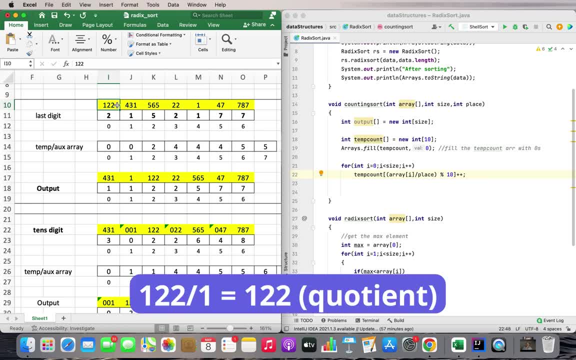 place will be 1.. 122 divided by 1 is going to yield the quotient as 122.. When 122 will be divided by 10, it's going to come out as 2.. All right, So the last digit is correctly calculated And in the 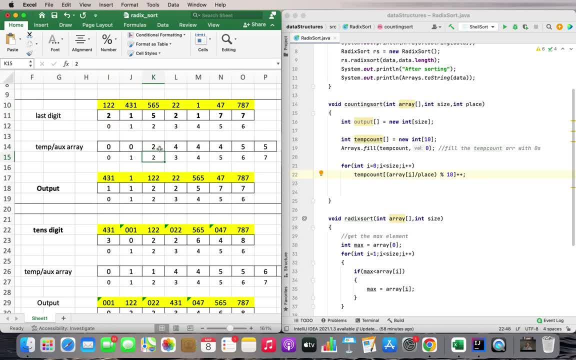 temp count array at index 2,, the value will be incremented by 1.. Okay, In the second iteration the value of the place variable is going to become 10.. So let's consider this number. For example, 431 divided by 10 is going to yield the quotient as 43.. When 43 is further divided by 10,, 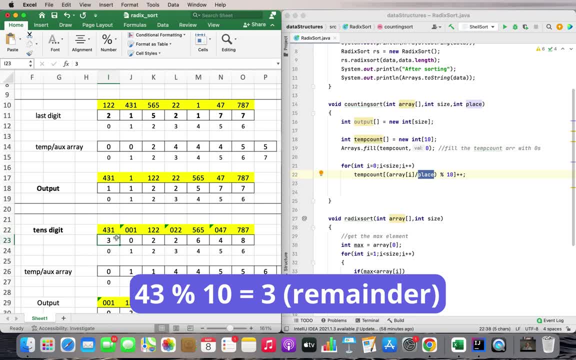 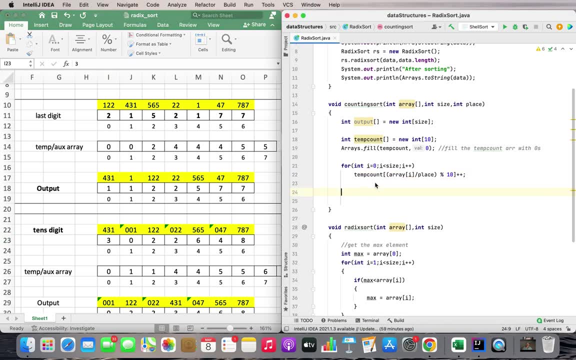 the remainder is going to come out as 3.. Hence the 10th digit gets correctly calculated by this code expression. Okay, Now we will modify the temporary count array to store the cumulative count, So the code for that will be another for loop, And this time it's going to start from 1.. 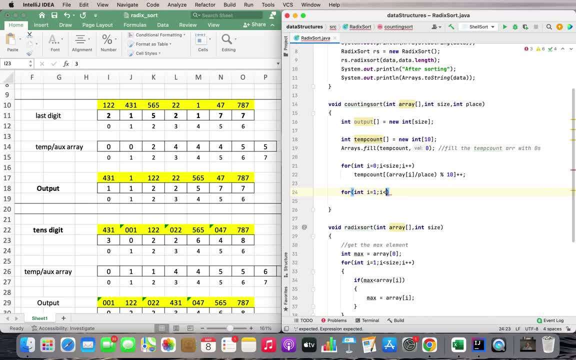 It's going to run till index 9.. So it will be i less than 10, i increment operator and within for loop we are going to write: temp count at index i equals to temp count at index i plus temp count at index i minus 1.. All right, This is going to modify the temp count. 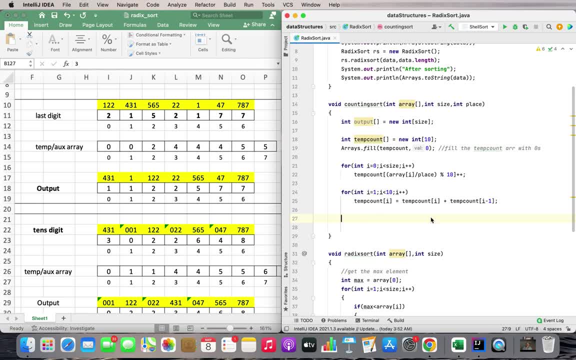 to store the cumulative count. Now we'll write the final step of the program, final step of the counting sort algorithm, in which we are going to place the elements in correct order in the sorted array. So it will again be a for loop That's going to start from the rightmost element. 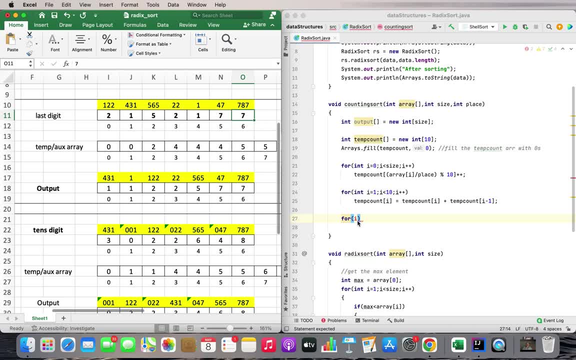 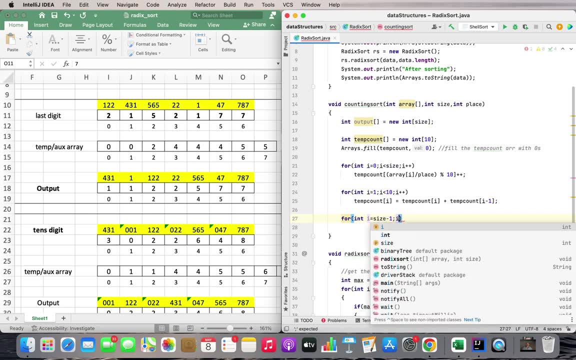 because that's what we have been doing, right. So it will be: int. i equals to size minus 1, and it's going to run till the first element, That means till index 0.. So it will be: i greater than equals to 0, i increment operator. All right, Since I have to place the elements in the output. 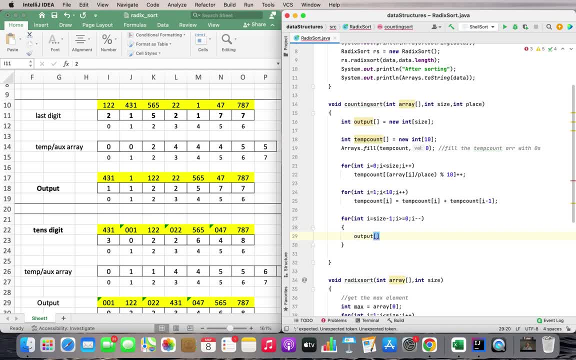 array. so it will be output and within square brackets we'll have to write some code expression. What will that be? So during our algorithm study, we picked an element from here, looked it up in the temporary count array to find the value. So this expression over here. 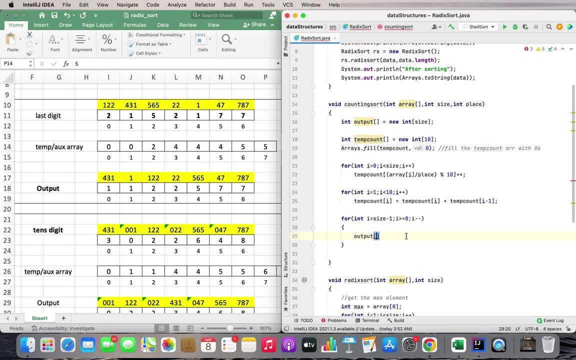 is going to do the job for us, So I'm going to copy it and paste it over here. Once we got the value, we subtracted 1 from it to get the index of the output array. Okay, So I'm going to subtract 1 from this expression And at that index we placed the. 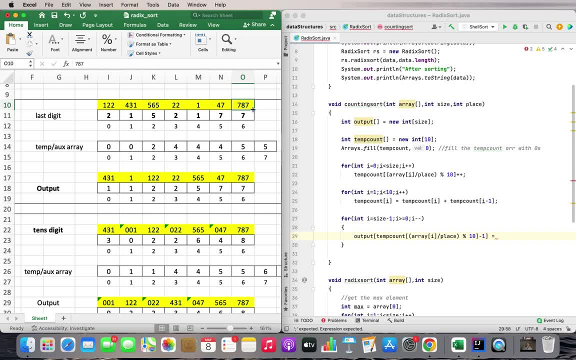 element from the input array. So here we are going to place directly the number rather than the individual digit. So it will be array within brackets. i Okay, And of course we updated the corresponding cell of the temporary count array with the decremented value with the value that. 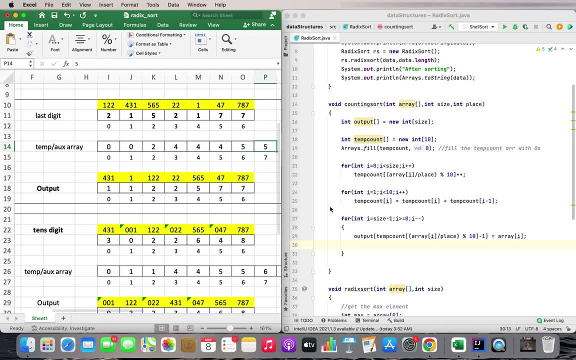 we got By subtracting 1 from it. Okay, So it will be this expression. I'm going to copy it. paste it over here and decrement operator. All right, The final step will be to copy the elements of the output array into the input array, So it will again be a for loop. It's going to. 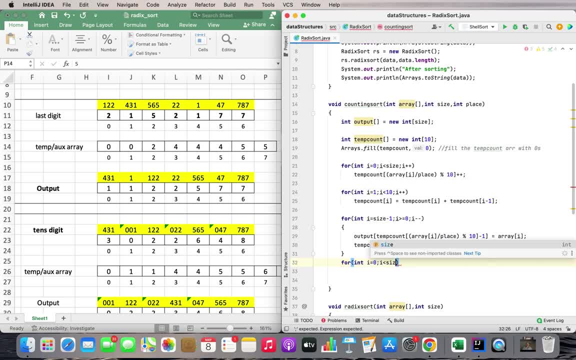 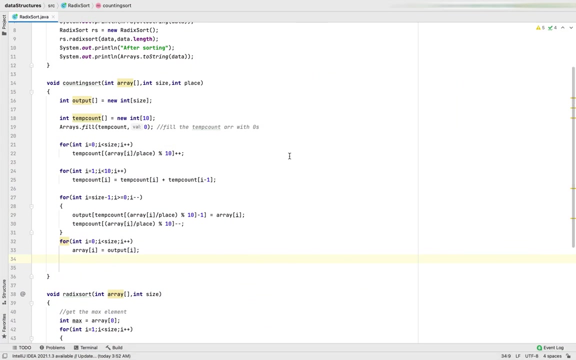 start from 0.. It's going to run for the length of the output array And within the body of the array, which is our input array, add index i equals to output array and index i. This will do the job for us All. right, I think we are done. Now let's run the program and check the output, Whether this 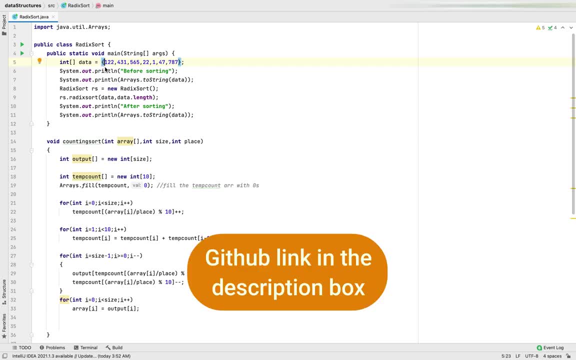 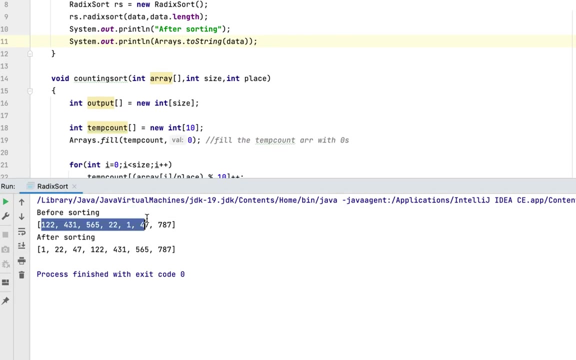 Java program that implements the radix sort algorithm is able to sort this array or not. And there you go. The array before sorting is our problem array. And look at this. This is the sorted version of the problem array, sorted in ascending order using the radix sort algorithm. 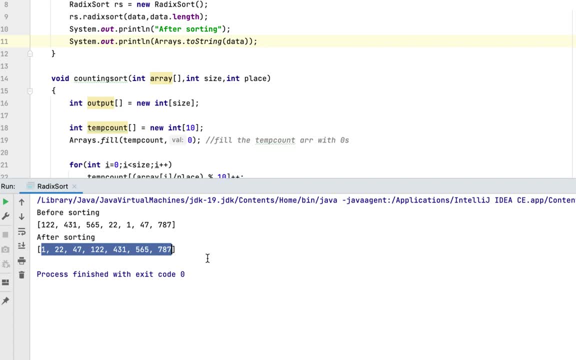 That means the program, the Java program implementing the radix sort algorithm is working pretty fine. By the way, you can find the GitHub link to this Java program in the description box of this video, And if you want to see the GitHub link, you can find it in the 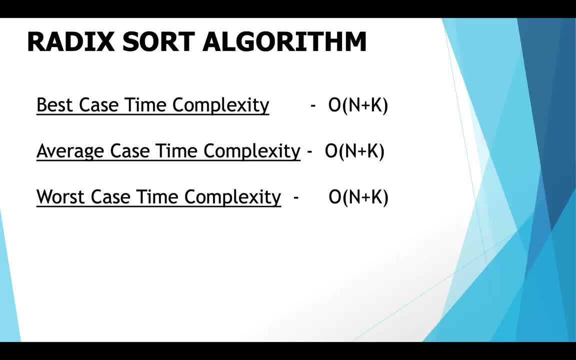 description box of this video. You can surely check it out. Let's now learn the time complexity of the radix sort algorithm. So the best case- average case- and the worst case- time complexity of radix sort algorithm is big O, n plus k And when it uses counting sort as the intermediate. 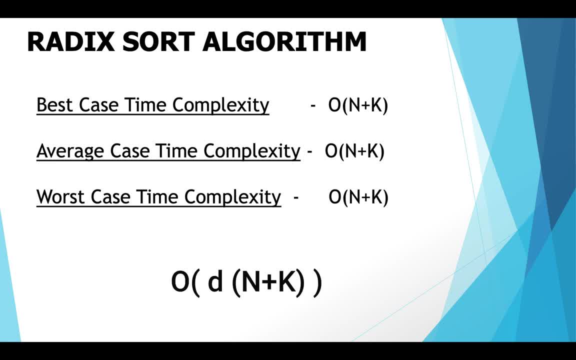 sorting technique. then the time, complexity becomes this: where d is the number of digits. With this we have come to the end of this video. I hope you enjoyed learning the radix sort algorithm from joeystech. To watch all the videos of joeystech, click the link in the description box.